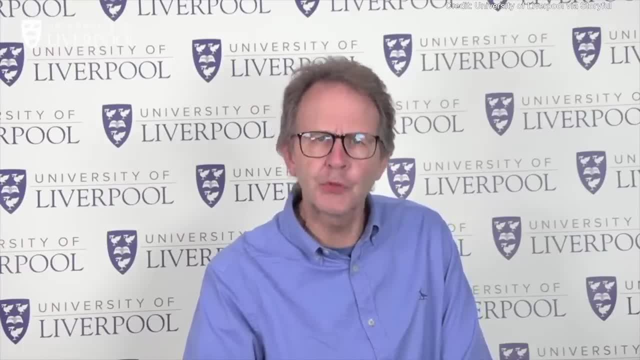 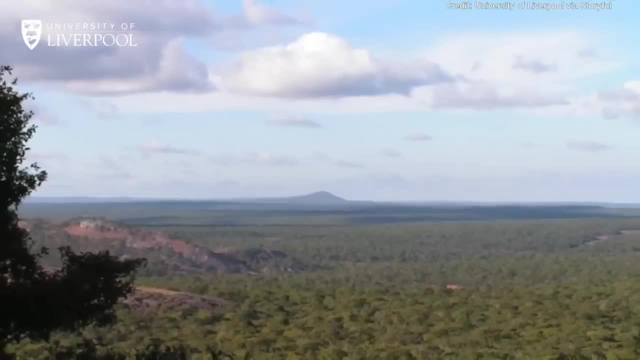 mean in terms of our understanding of early humans. So join me on this journey. Before we visit the excavation, I'd like to introduce you to the woodlands of Zambia. This part of Africa is blanketed in a beautiful tropical woodland as far as the eye can see. The woods are important. 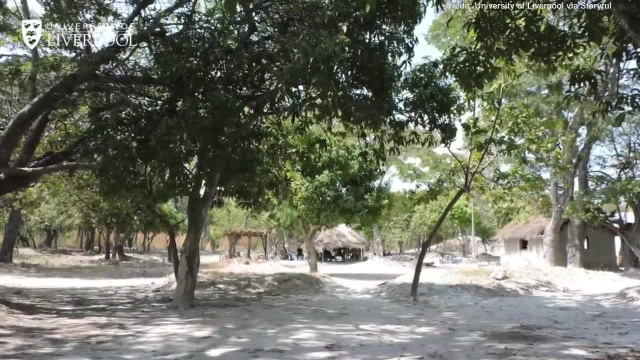 today, as they are important for the environment. The woodlands are important for the environment. The woodlands are important for the environment. The woodlands are important for the environment Today, and they probably were important in the past. Woods can give you fuel for making a fire. 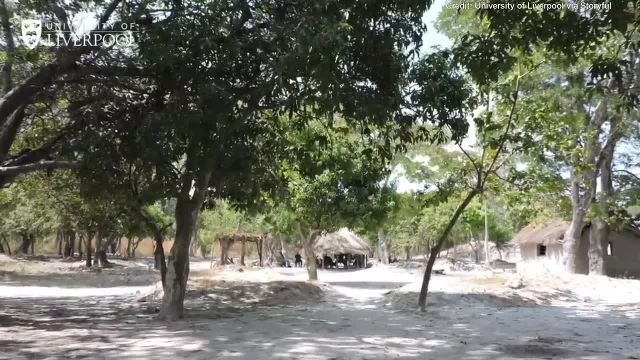 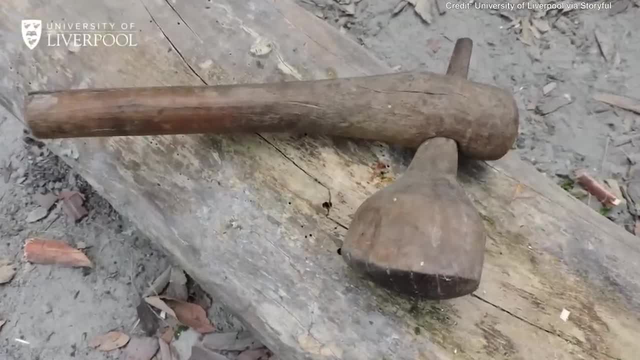 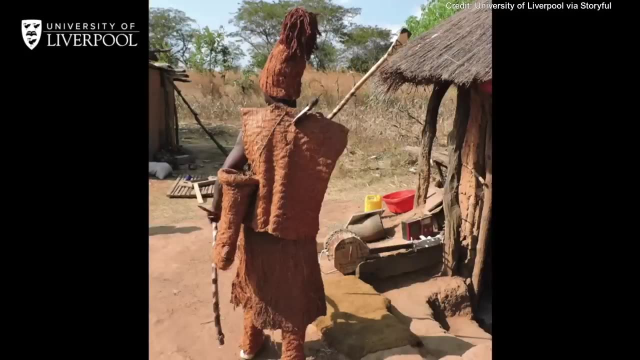 They can provide food in terms of nuts and fruits. You can make shelters or huts. You can make tools of wood, and the bark and the leaves provide medicine and even clothing. The bark can be stripped into clothing. That's a traditional cloth you're seeing here which is no longer being made. 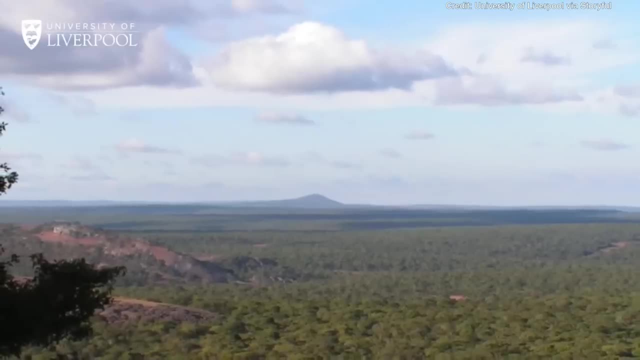 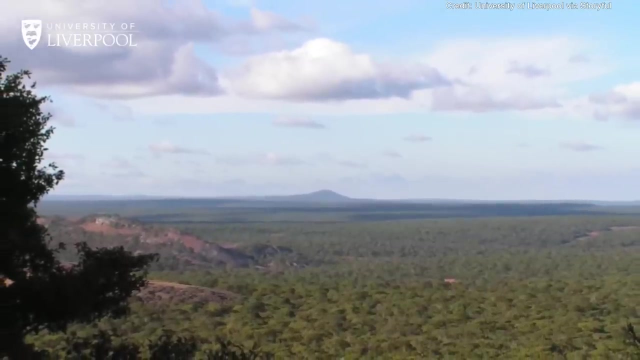 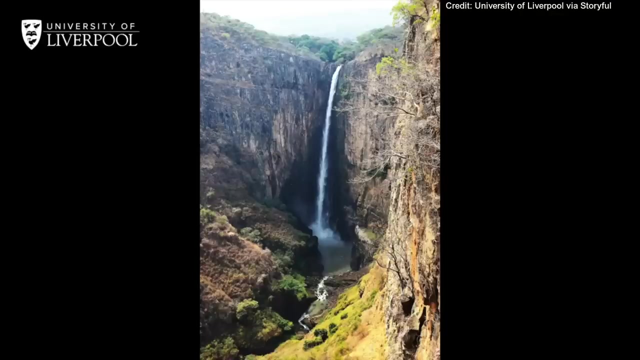 It's a dying art. So if wood is so useful now and has been in the past, why aren't we finding evidence of it in the early archaeological record? And the answer lies in the fact it's just not preserving, except in places like Colombo Falls. This is the majestic Colombo Falls, more than 230 meters high. 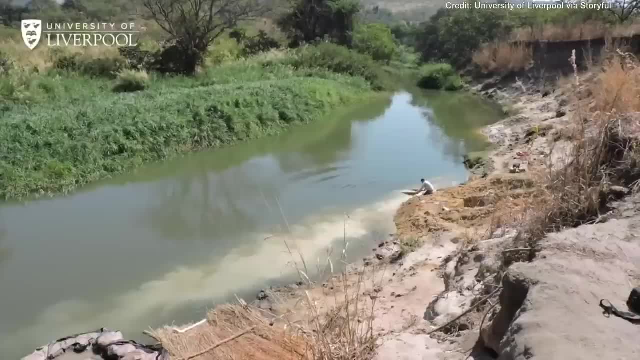 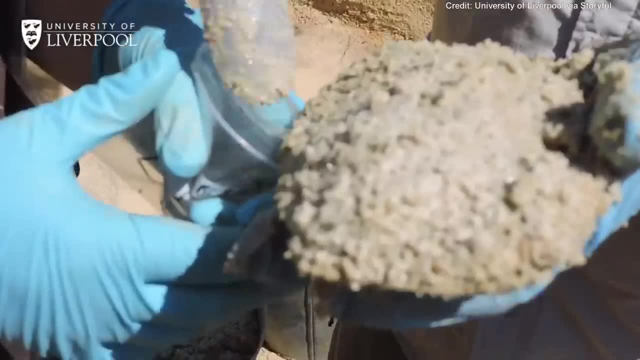 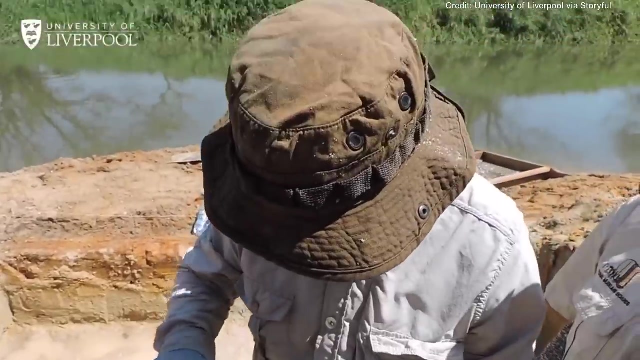 second highest falls in Africa. but the important thing is what's behind it. It's the Colombo River and a basin which preserves the archaeological record, including wood. Here you see students excavating one of the early sites. We're finding the tools that were used, or the kind of tools that were used, to make and shape the wood, and you can see a little. 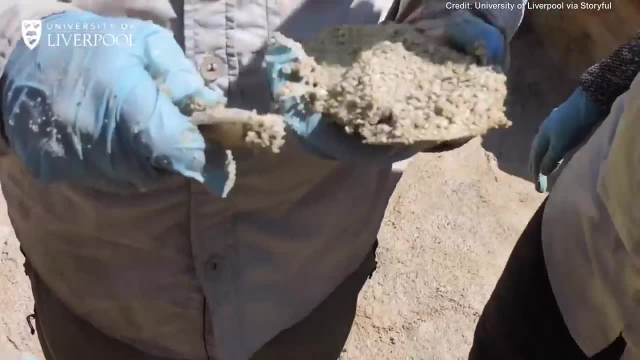 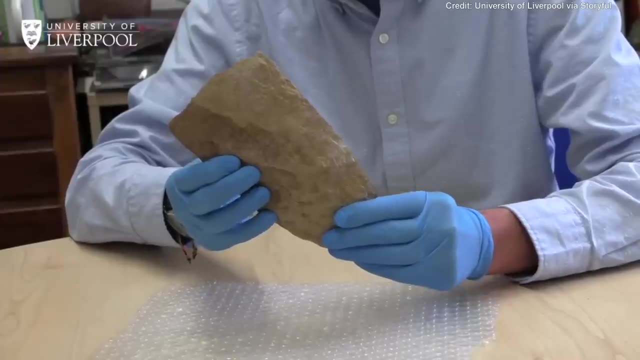 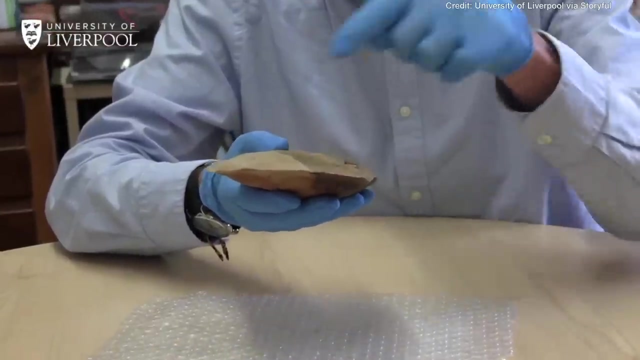 bit of the river as we move along. This object here is being excavated with a plastic tool so it doesn't damage the edge, and so we can study how it was used. This is a cleaver. It's got a strong, broad edge. You can see it curves just a little bit and it's an excellent tool, we think, for working. 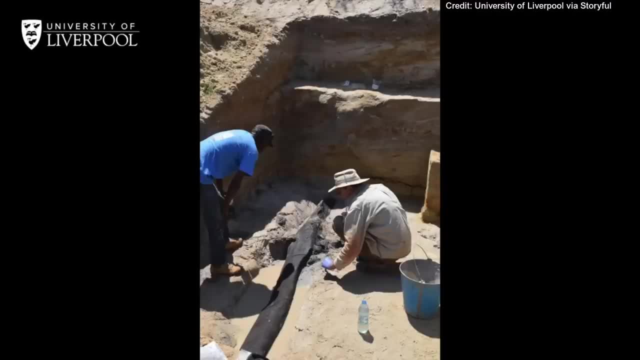 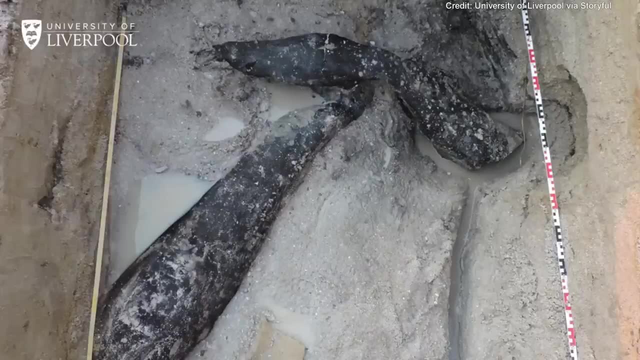 hard materials like wood, and you can see here a large tree trunk, And beside it, where I'm sitting, comes this wedge shaped object. It's a tool. The most important objects, though, are these: These are overlapping pieces of wood. When we found them, we thought this: 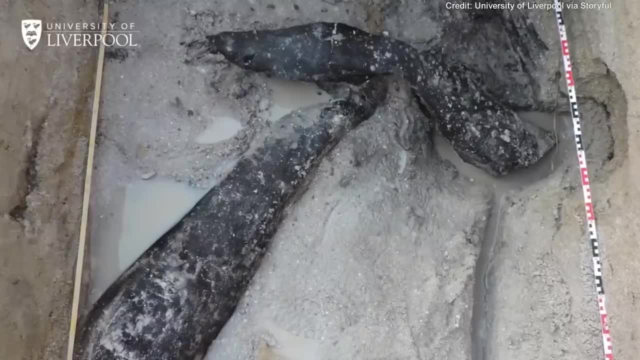 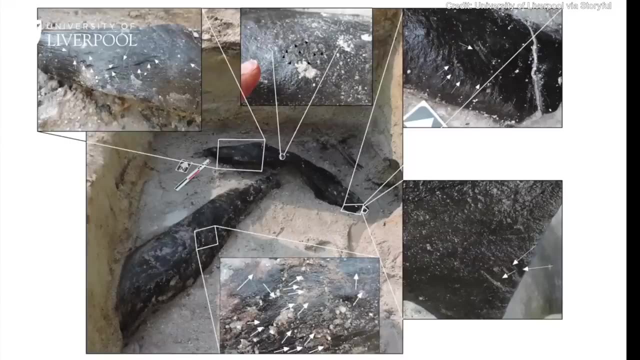 was an unusual arrangement and as we started to look at them, the piece on the top has a notch in the middle. That notch has been cut, The ends either side of it have been tapered and it sits on a tree beneath, But again, it's not just any tree. 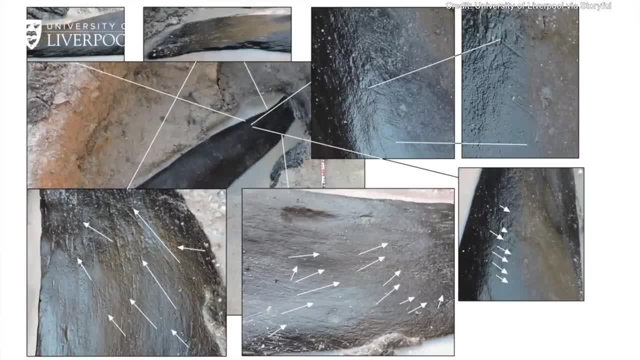 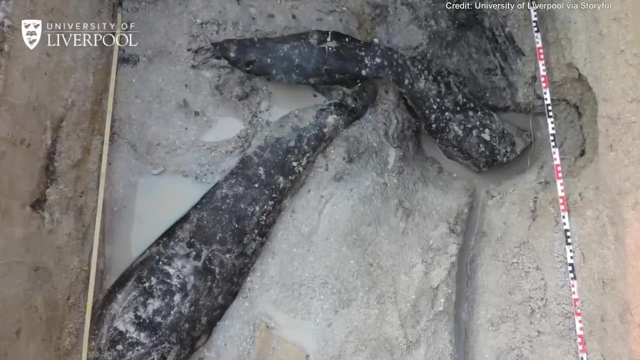 The tree also has been shaped. The pictures here show the white arrows, and each of these is a mark left by a stone tool. They could be scraping, they could be chopping. They're all involved in making those two pieces fit into what is the world's oldest structure We are looking at. 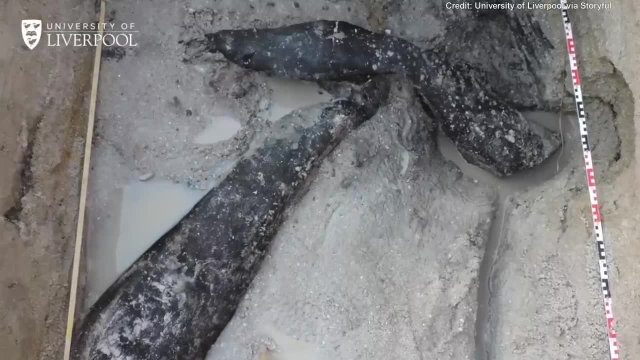 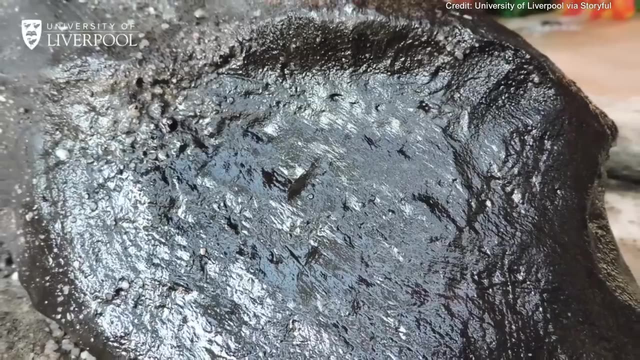 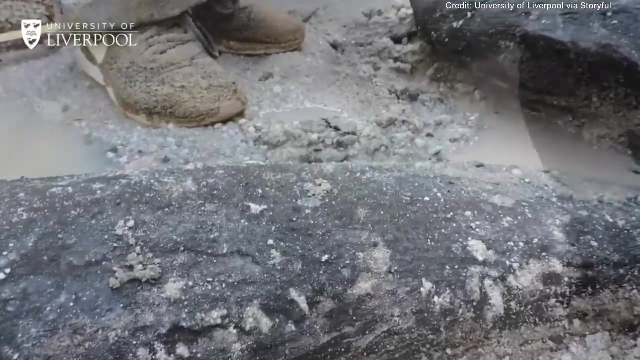 something more than 477,000 years old here, Almost from the moment of discovery, we had to keep the wood wet, Keep it from drying out, from cracking and from losing the signs of the human working on the wood. Back here in Liverpool we have tanks specially designed for underwater photography to 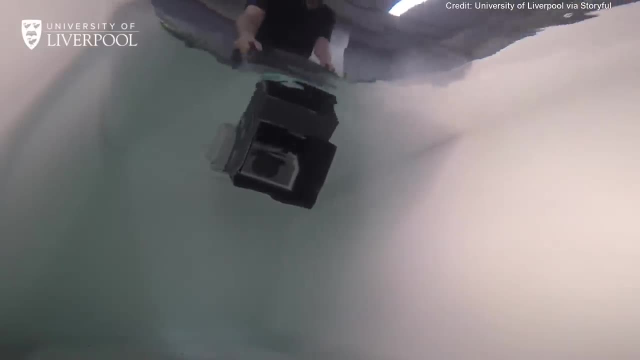 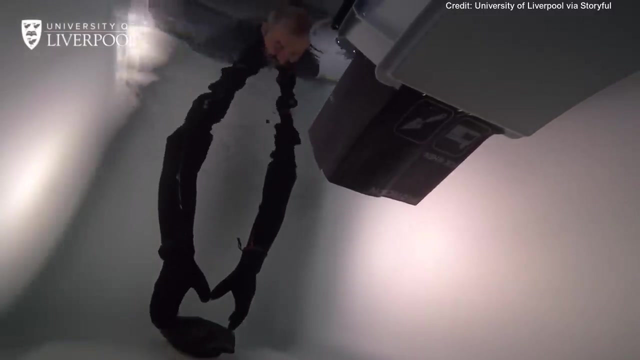 build 3D models of the wood. You're seeing the camera, specially developed, and the first piece that's being examined here is the wedge. Do you remember the wedge near the big tree trunk? Well, here the hands are coming down holding the wedge, turning it around. Photographs are being made. 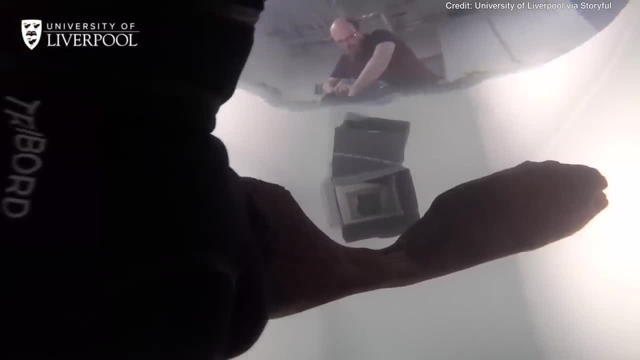 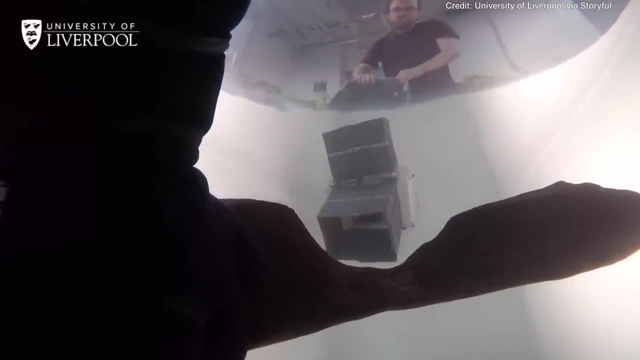 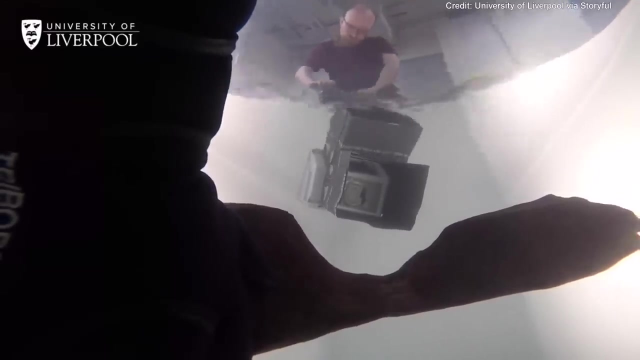 Next we're seeing a part of the structure. This is the centre section. The structure is now in three parts. It was naturally cracked over time and this is the middle part. with the notch You're seeing JR, He's photographing it in all sorts of different. 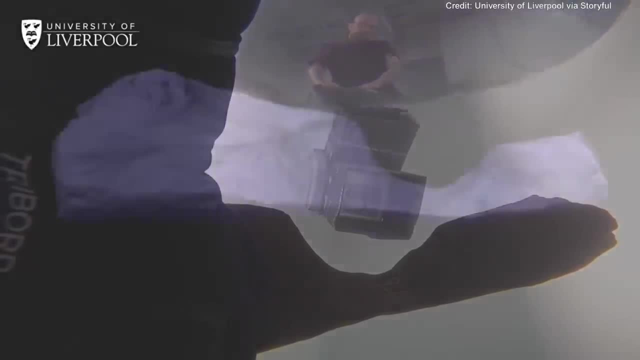 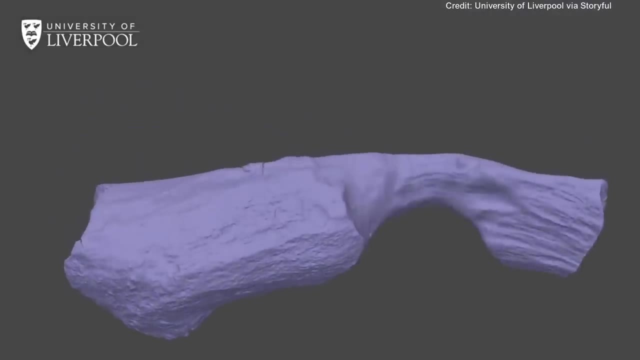 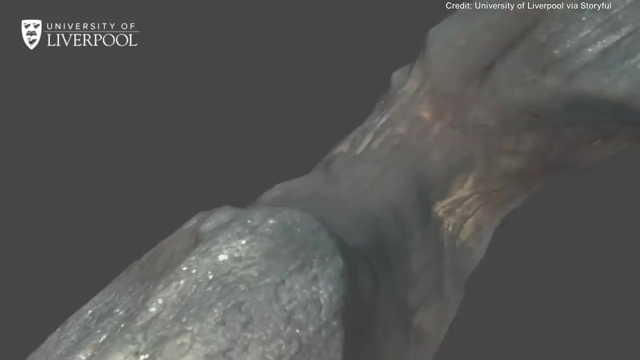 directions building the three-dimensional model. And here it is the model. We can turn it over. You can look closely at the notch And now we have the colour And I can see the cut marks on it. I can see where the wood has been removed. That's an important piece. 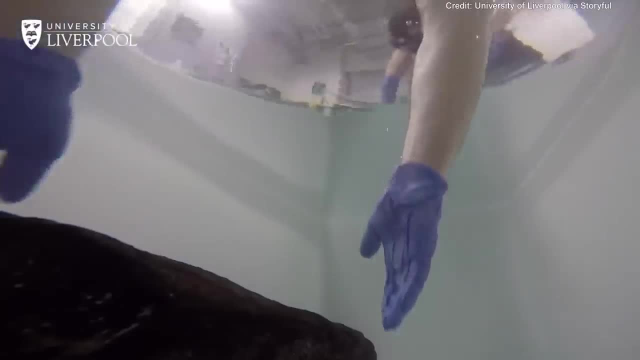 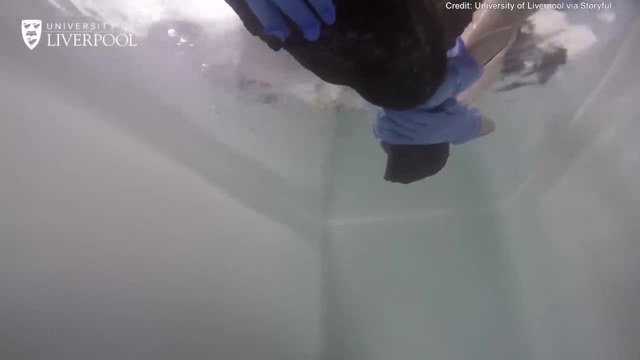 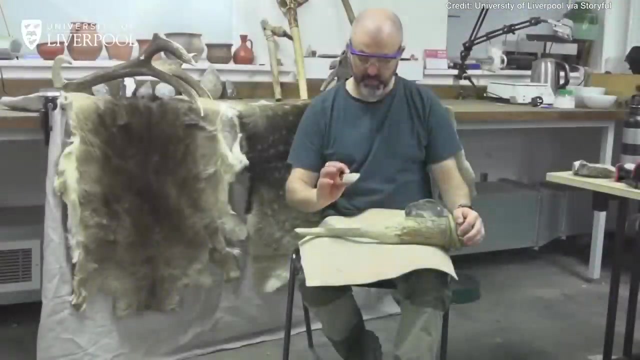 And once we've finished the analysis, we lift it carefully, removing it from its photographic bath and putting it into its storage bath. It's heavy, It's solid And the wood is now being conserved. So once we have made the 3D models, we need to understand what those marks are telling. 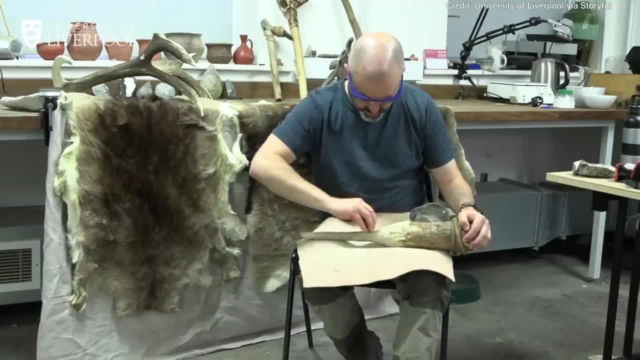 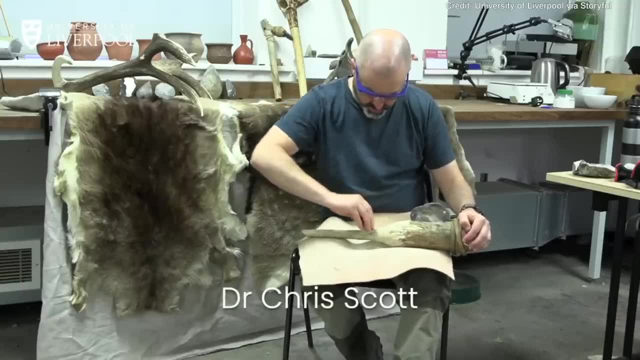 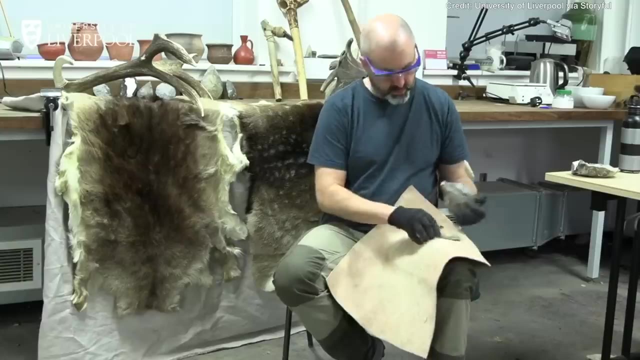 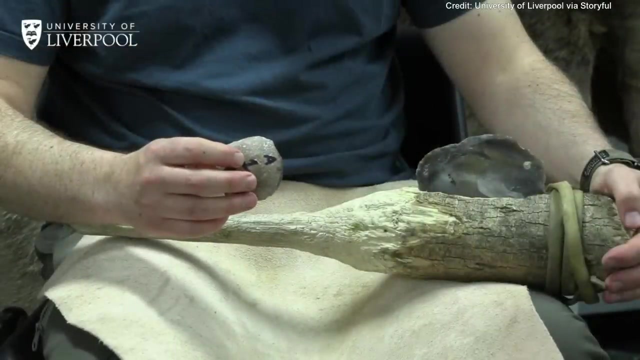 us about the tools that were used and how they were used, And to do that we need experimental archaeology. Here in Liverpool we have our own ancient technologies workshop And Chris here is an expert in making and using stone tools. He's making a flake of stone and he's going to use a stone which we found at Colombo Falls. It's 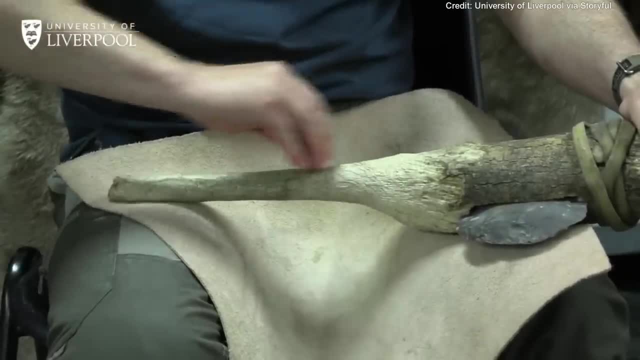 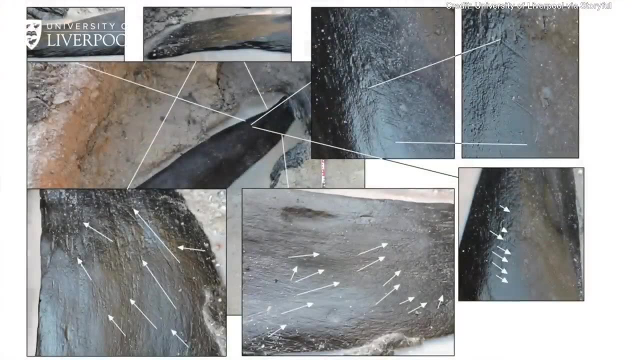 the same raw material And he's going to use that to shape a wooden handle and seeing what kind of marks the stone leaves on the wood. We can then take those marks as a reference and look at the prehistoric wood- And yes, we do. 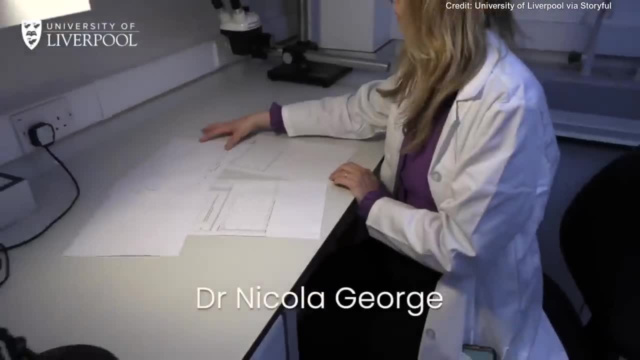 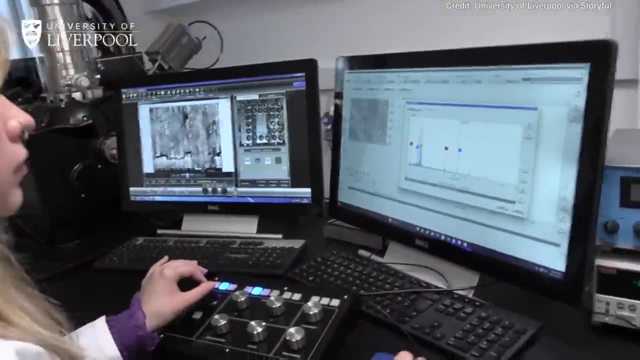 find very similar marks from scraping. In our labs in Liverpool we also have a variety of different kinds of microscopic techniques of analysis. Nikki here is looking at the surface of the wood for any evidence of changes from fire. Our research has shown not that there is direct evidence of fire. 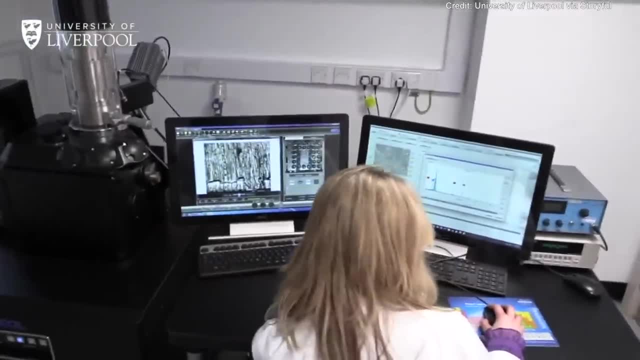 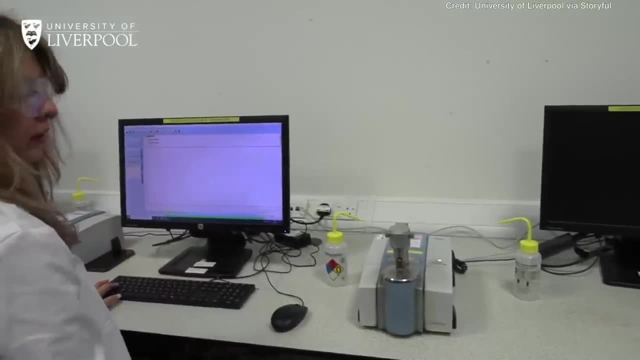 it may be there, but that's going to be something to examine in future work. But we do have evidence that the wood is partially fossilized. By that I mean minerals. silica minerals dissolved in the water have actually entered the wood and replaced some of the wood structure, So that's given the wood some. 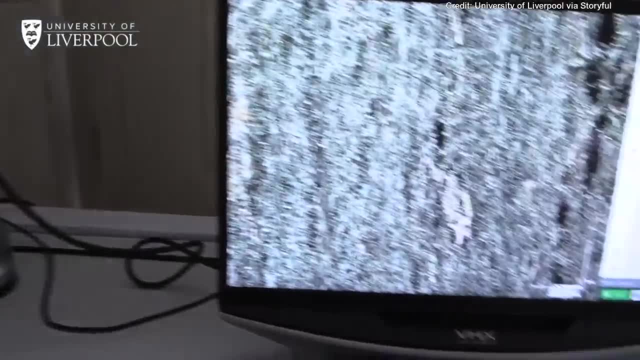 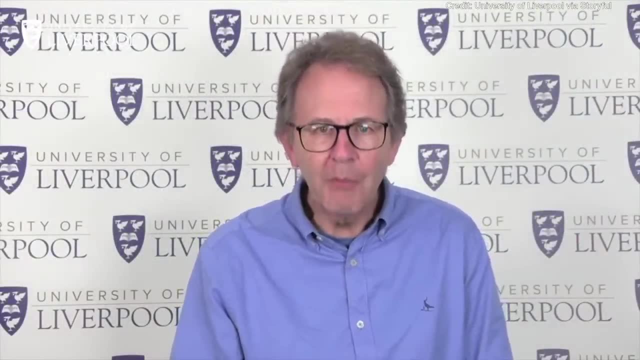 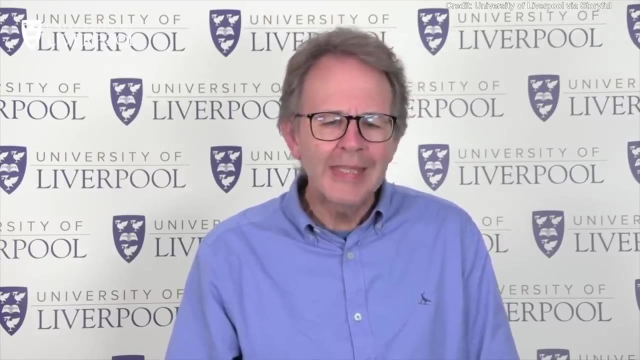 strength that's helped it survive all these hundreds of thousands of years. We know how old the wooden objects are, we know how they were made, but the structure, it's a real enigma. What was it used for? It's not something we're. 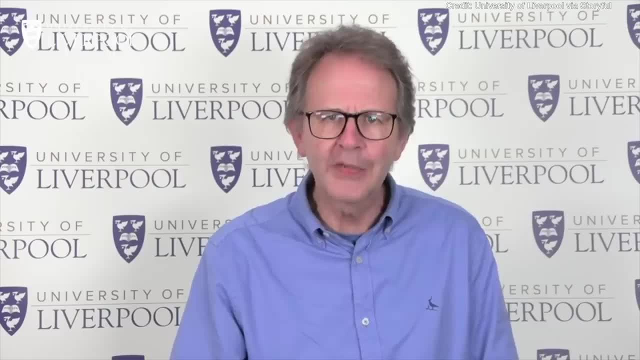 familiar with today. it doesn't look like what we might think of as a structure, But we have to ask: what is a structure? What's things that, combined as a framework, they support something? Okay, once we have that idea, then we can start to think maybe what was it used for? How was it built? And to 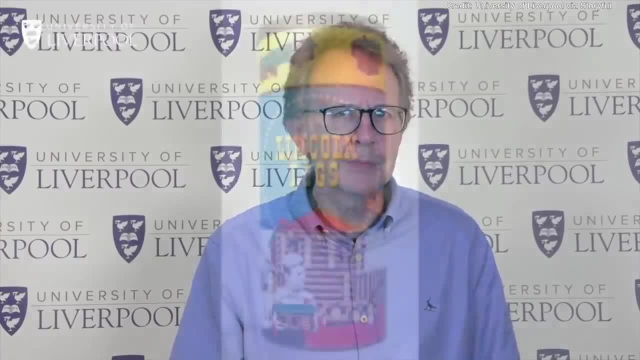 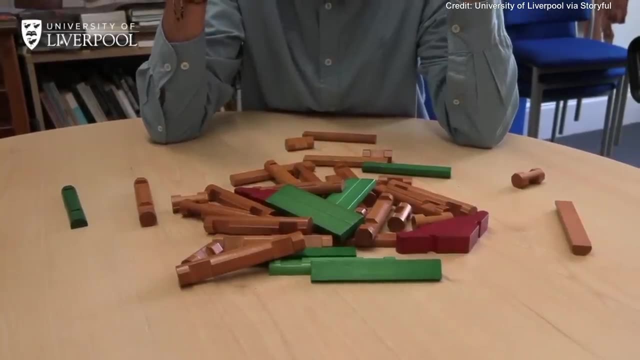 help me think about this. I turned to a childhood toy When other kids were playing with Lego. I was in my room making log cabins from Lincoln logs and I don't know why they came to my mind, but they did and they have. 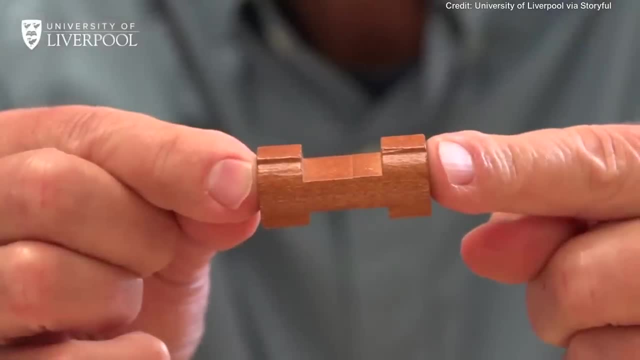 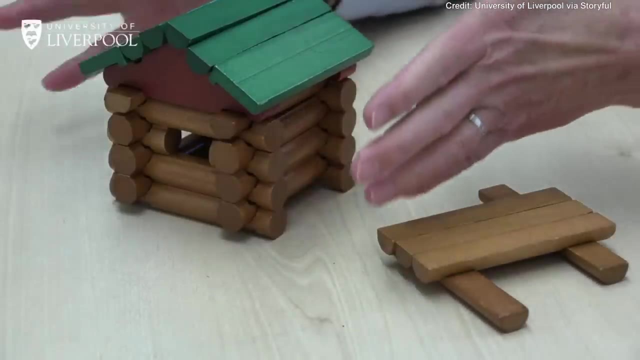 helped me think about the Colombo Falls structure. What's the big deal here? Well, Lincoln logs have a notch in them and the notch allows one piece to sit on top of another and you can build things with this. You can build log cabins, but I'm